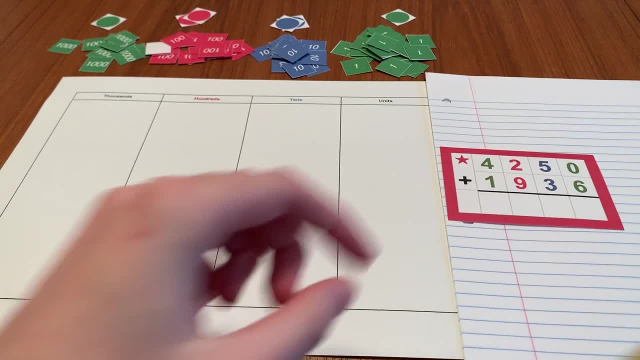 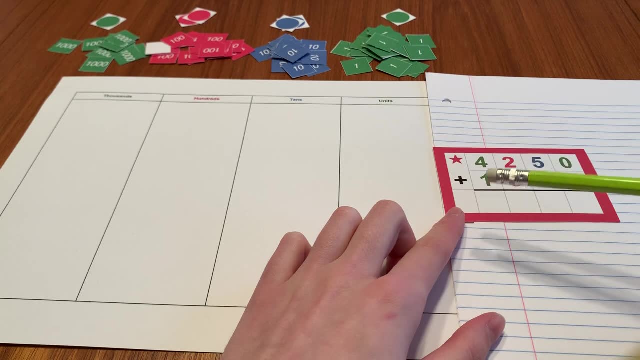 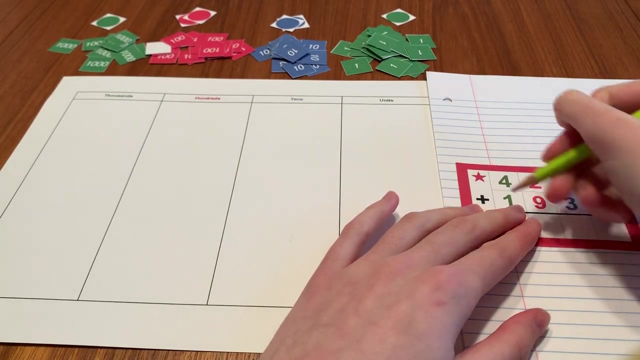 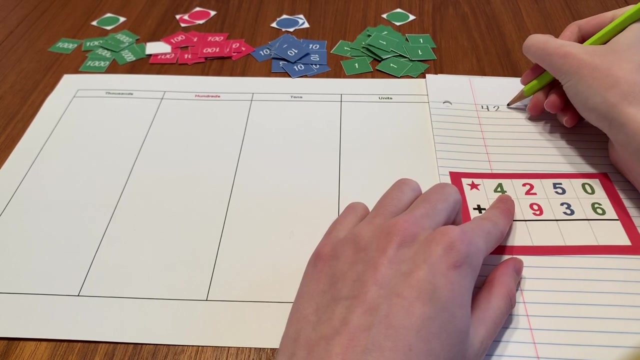 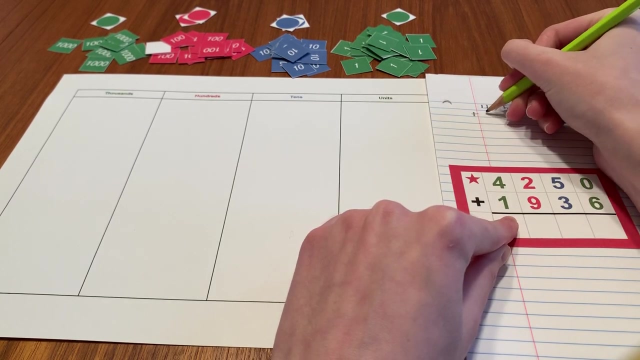 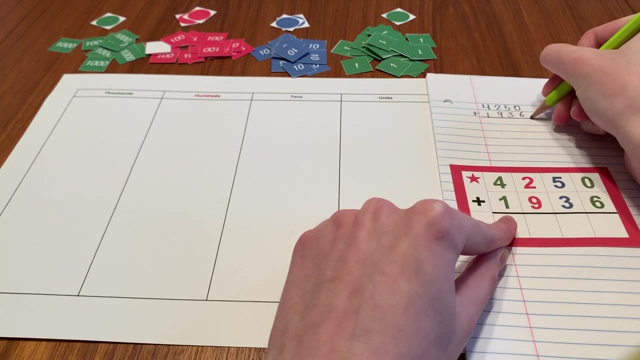 This is addition with the stamp game. So this star means that this will be a dynamic addition problem. That means that we're going to regroup or make an exchange. So we're going to start by writing this problem on this paper: 4,250 plus 1,936.. And then I draw this line here. So I'm going to start by making the first. 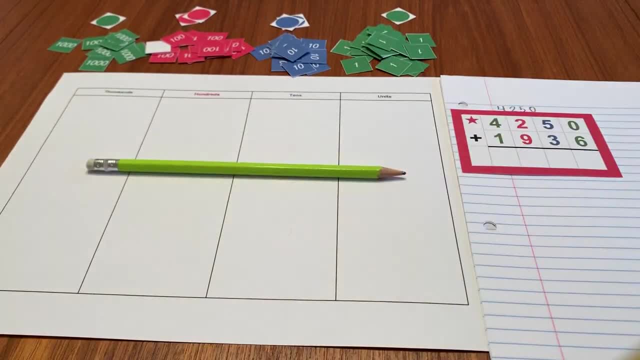 number 4,250.. So I always like to start in my units place. And because there's 4,250, I'm going to start by making the first number, 4,250.. And then I draw this line here. So I'm going to start by making the first number, 4,250.. And because there's 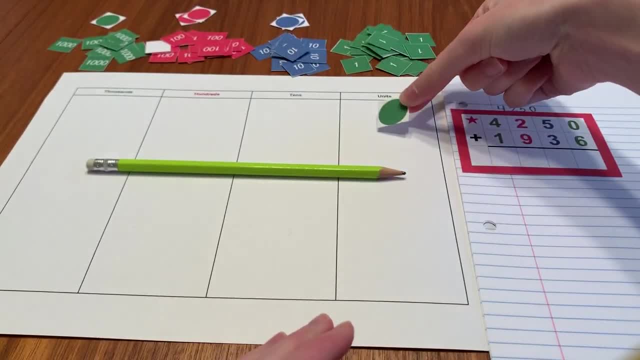 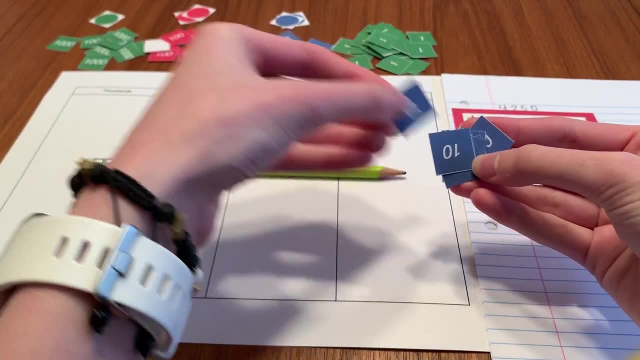 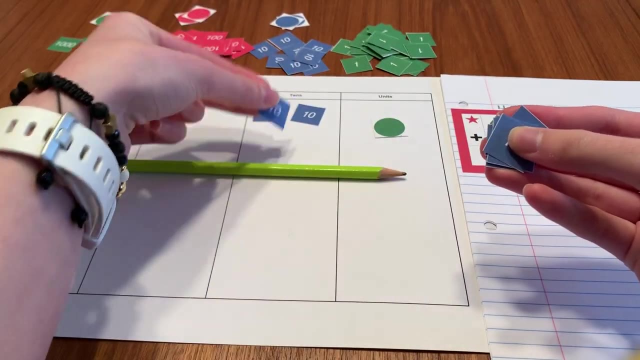 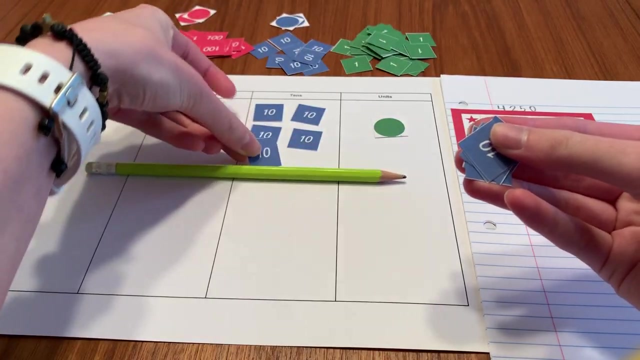 a zero there. I'm going to use this circle as a placeholder. Now I go to my tens. I have five tens. Five ten, twenty- I was about to start counting by fives- Thirty, forty and fifty. Five tens makes fifty. Now I go to my hundreds and I have two hundreds. 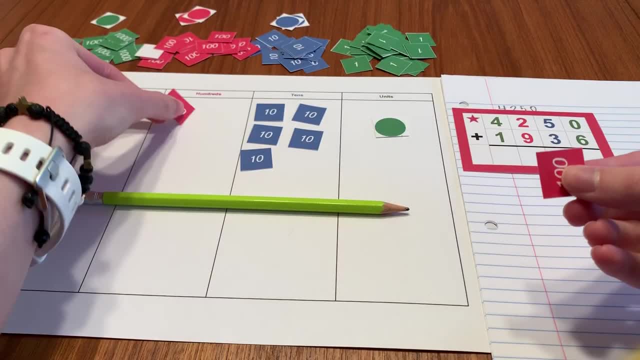 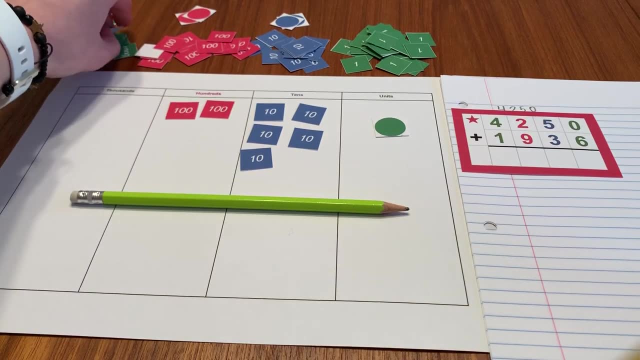 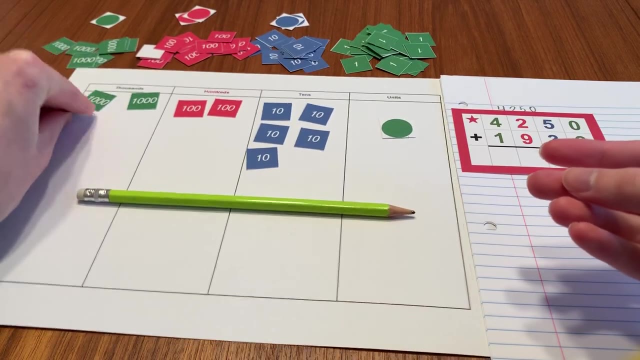 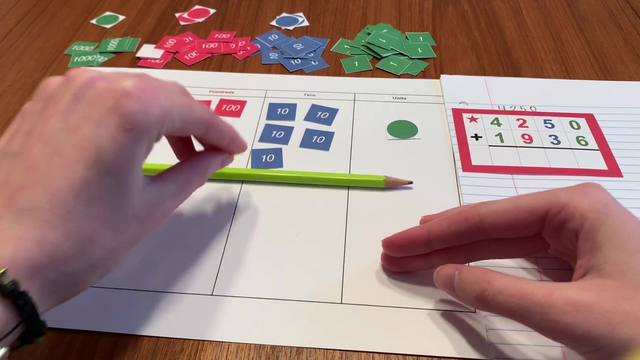 in this number, One hundred and two hundred, And then in my thousands place I have four thousands, One thousand, two thousand, three thousand and four thousand. Now I'm going to be using this pencil as my placeholder for the next moment And 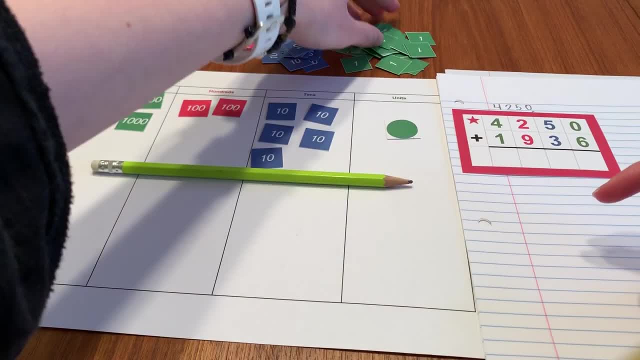 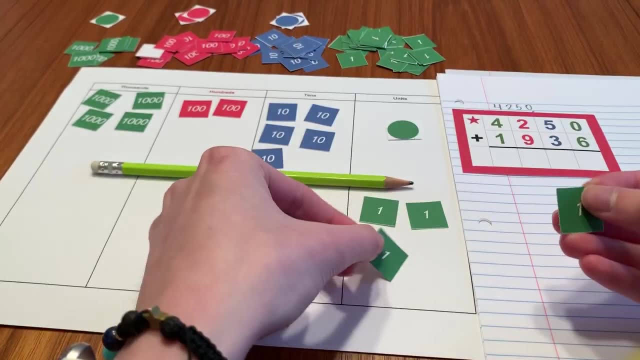 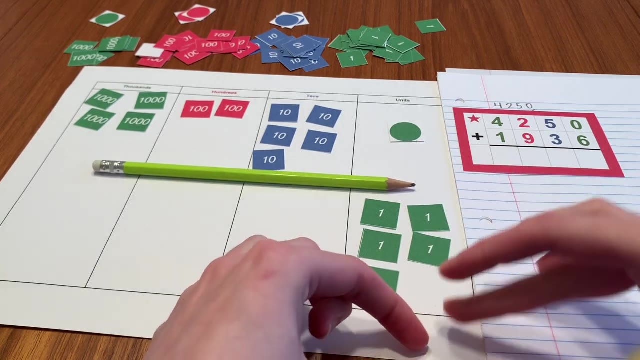 now I'm going to make the second number. So in my ones place I have six, Six units: 1, 2, 3, 4, 5, 6. These little paper ones are kind of tricky sometimes. 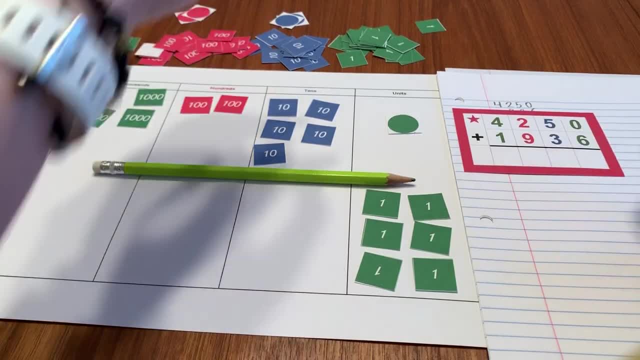 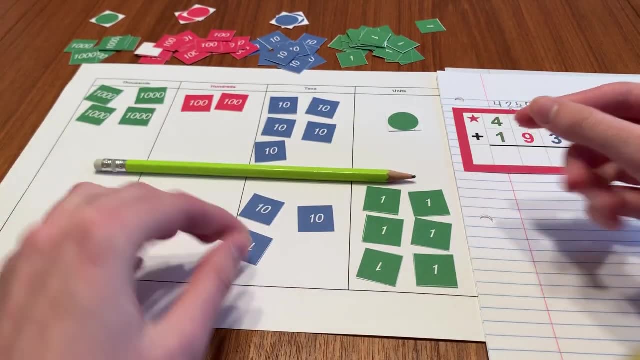 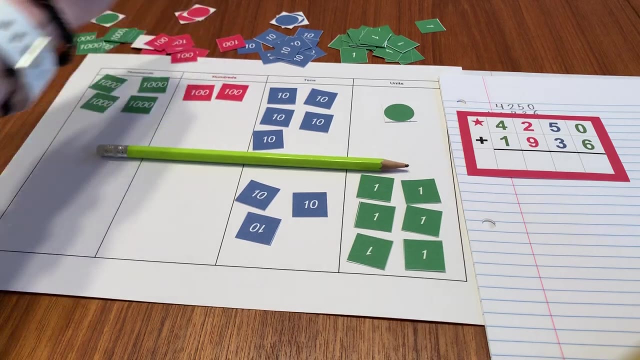 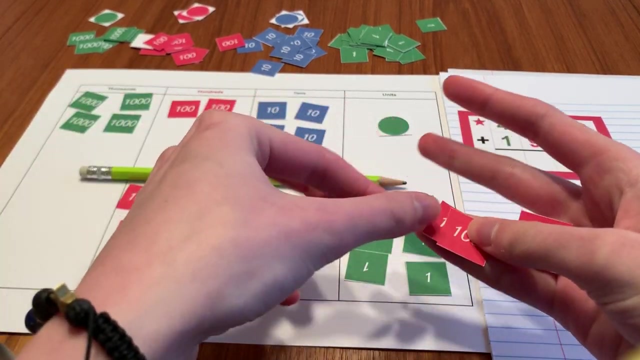 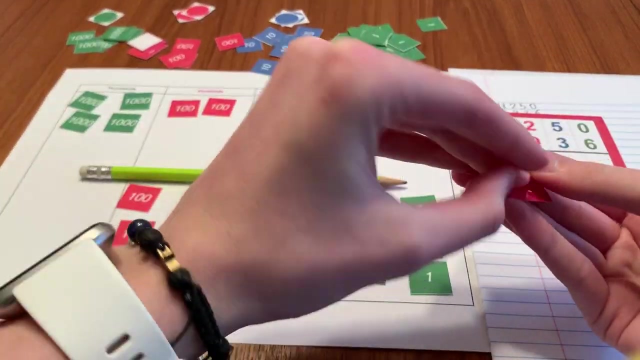 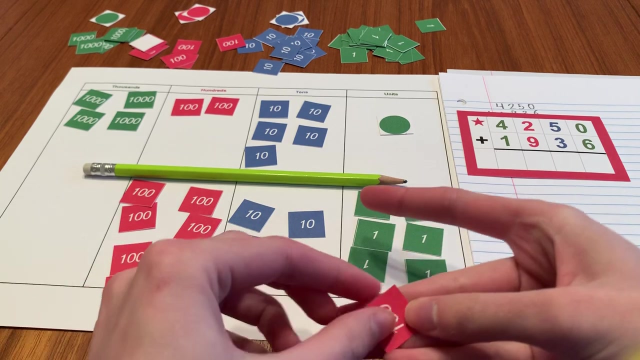 And then, in my tens place I have three tens: One, two and three. In my hundreds place I have nine hundreds, One hundred two hundred three hundred four hundred five hundred six hundred. I need three more hundreds: 800, 900.. There we go, Alrighty. And then finally, 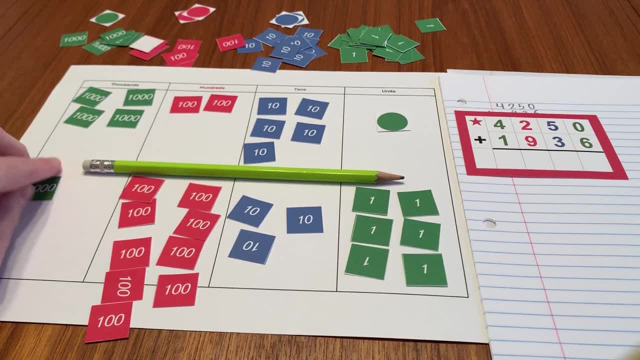 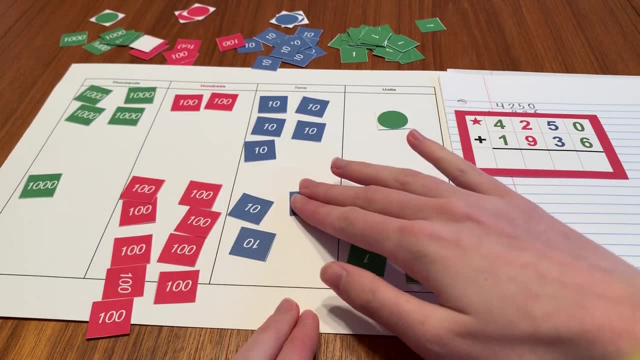 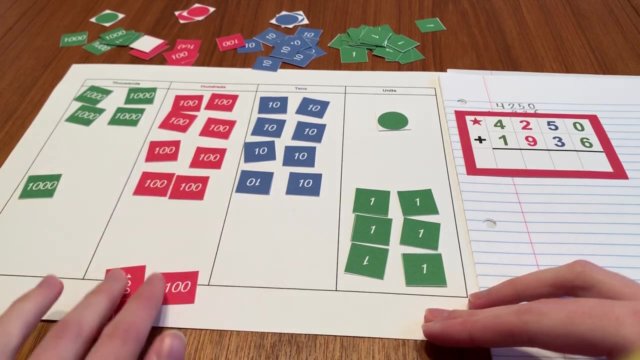 in my thousands place. I have four thousand, two thousand, three thousand and four thousand. So I have, I have 1000.. Nice and easy. So now I'm going to slide the second numbers up to combine them with the first number. I'm combining my two addends together to get my answer. 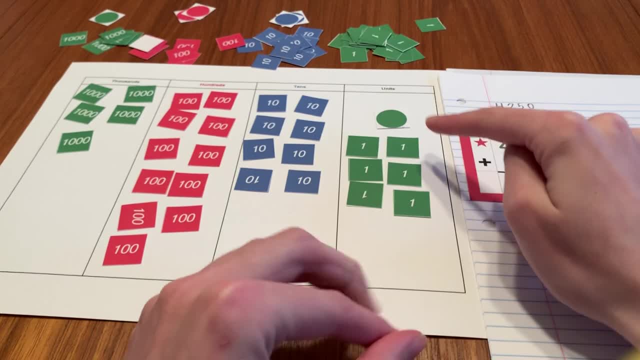 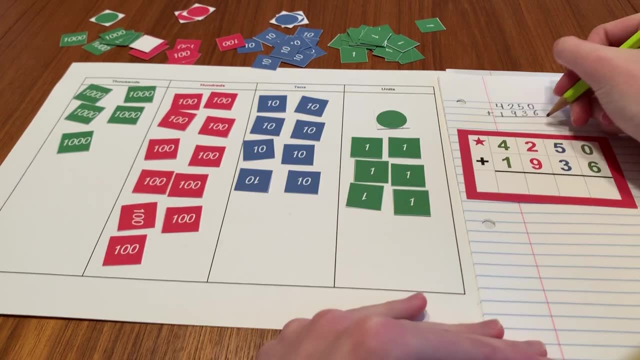 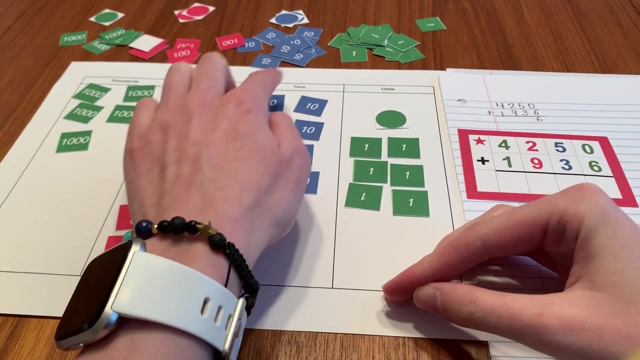 So I always like to start in my units place And I'm going to count them up: 0 plus 123456 equals 6.. Now I look at my 10s. I had 5 10s plus 3 10s, 10,, 20,, 30,, 40, 50,, 60,, 70,, 80. 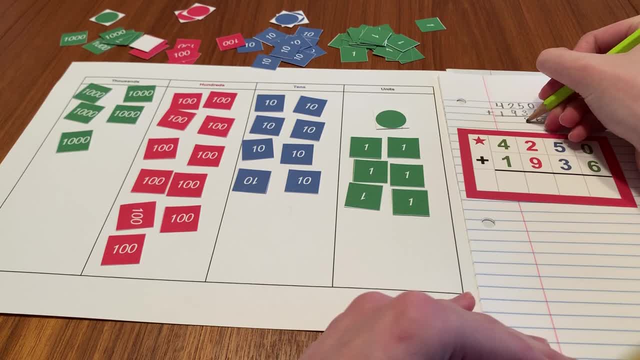 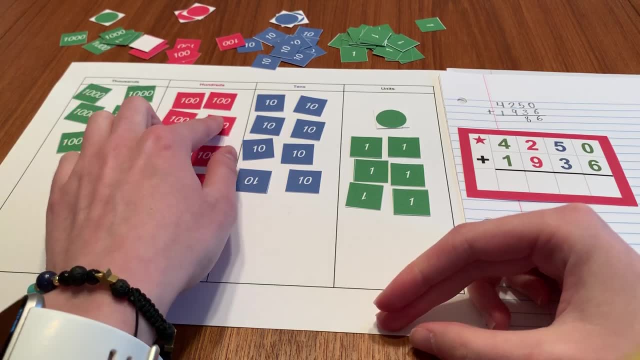 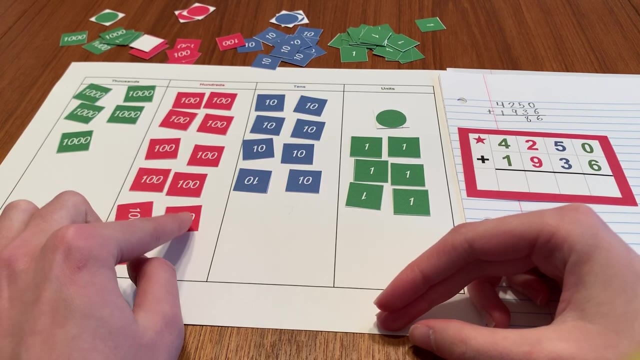 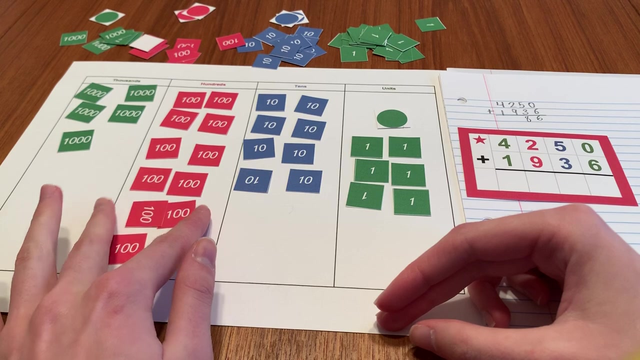 I have 8 10s. Now I'm going to count my hundredths: 100, 200, 300, 400, 500, 600, 700, 800, 900, 1000.. So that means it's time to make an exchange. So when I get to 10, I stop and I make one. 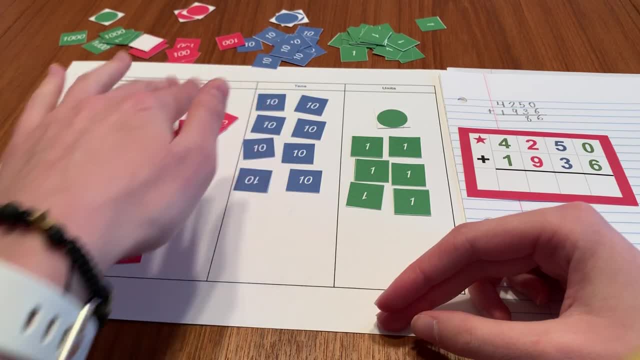 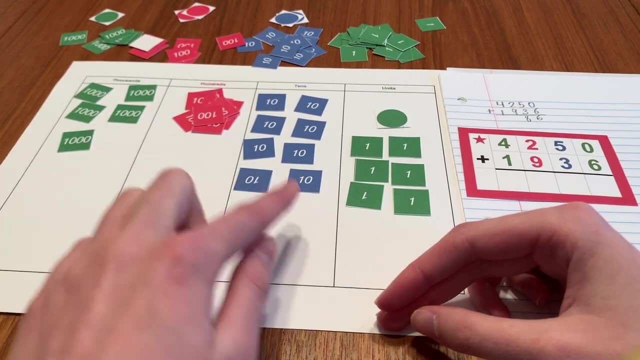 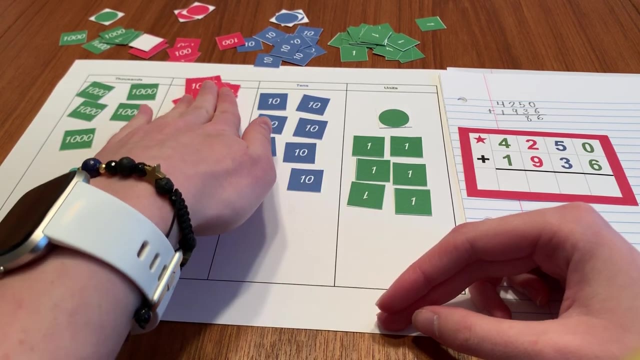 neat pile And I'm always going to trade it for the number 1 to my left. So 10 hundredths make a 1000.. 0. Just like 10 10s make a 100. And 10 units make a 10.. So I'm going to go to the bank. 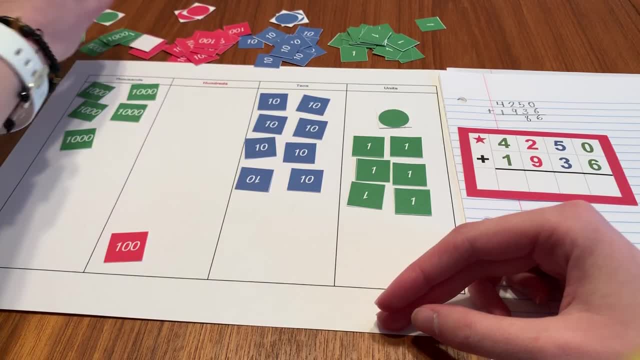 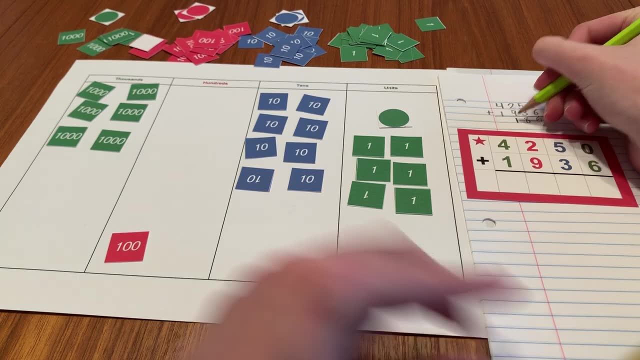 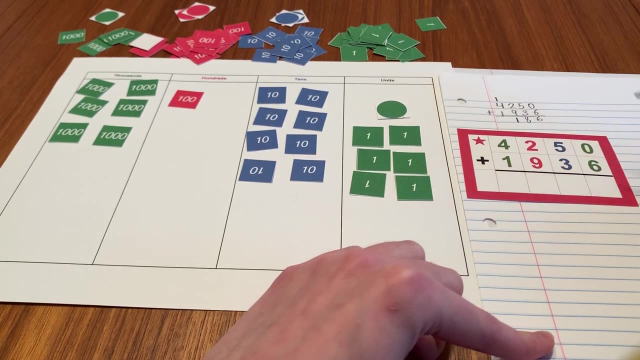 and make an exchange. I'm exchanging 10 hundredths for 1000.. And here's how I write that: I put a 1 here for my 100. that's left And I added I made a new 1000.. So that goes right there.